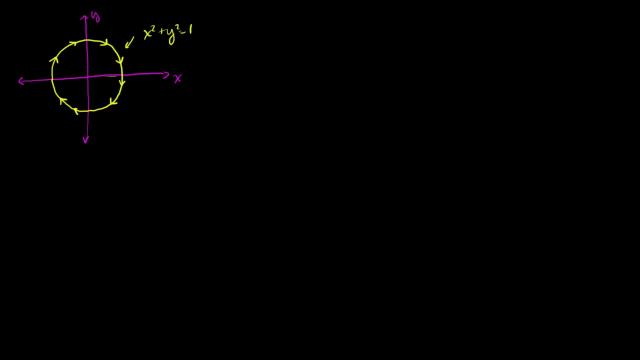 unit circle, And what we're concerned with is the line integral. the line integral over this curve c, over this curve c, It's a closed curve c, it's a closed curve c and it's actually going in that direction. So we have the equation of 2y dx minus 3x dy. So we are probably tempted to use Green's theorem. 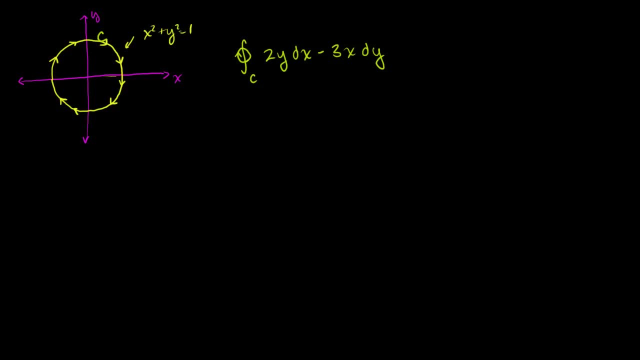 and why not? So let's try. So this is our path. So Green's theorem tells us that the integral of some curve f dot dr over some path where f is equal to where f is- let me write it a little bit neater- where f of xy. 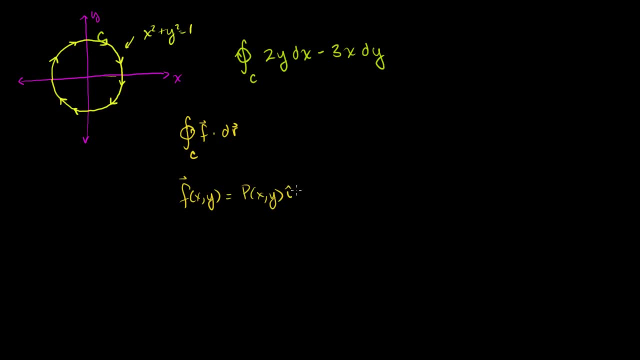 is equal to p of xyi plus q of xyj that this integral is equal to. it is equal to the double integral over the region- this would be the region under question in this example- over the region of the partial of Q with respect to X minus the partial. 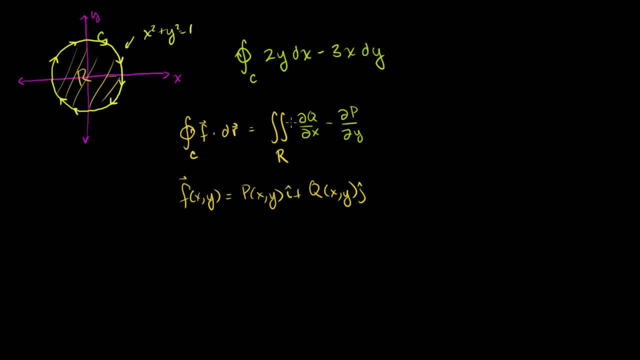 of P with respect to Y, All of that DA, the differential of area And, of course, the region. is that what I just showed you? Now you may or may not remember? there's a slight subtle thing in this which would give you the wrong. 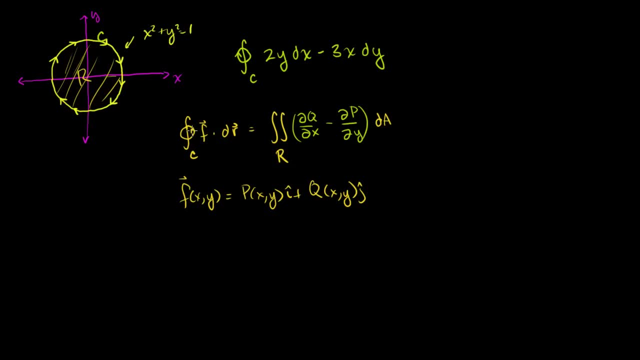 answer. In the last video we said that Green's theorem applies when we're going counterclockwise. Notice, even on this little thing, on the integral, I made it go counterclockwise. In our example the curve goes clockwise. 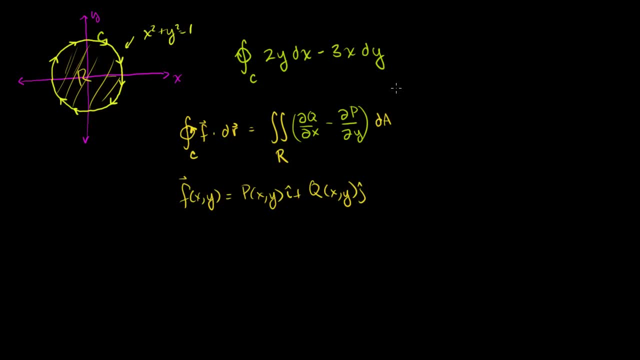 The region is to our right- Green's theorem. this applies when the region is to our left. So in this situation, when the region is to our right and we're going clockwise, so this is counterclockwise. So in our example, where we're going clockwise, the region is 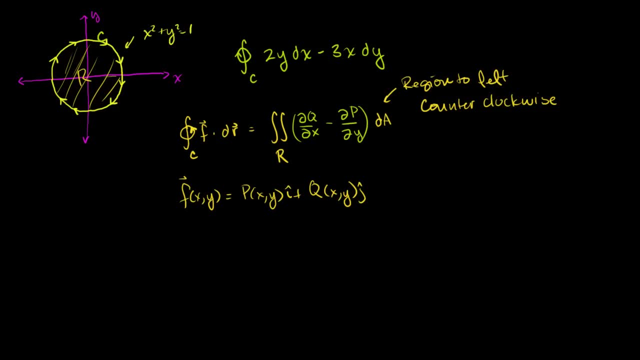 to our right. Green's theorem is going to be the negative of this. So in our example we're going to have the integral of C and we're going to go in the clockwise direction. So maybe I'll draw it like that of f dot dr. 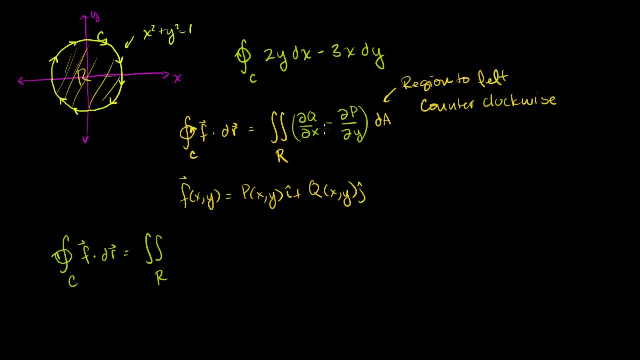 This is going to be equal to the double integral over the region, And we could just swap these two, the partial of p with respect to y, minus the partial of q with respect to x, da. So let's do that. So this is going to be equal to, in this example, the 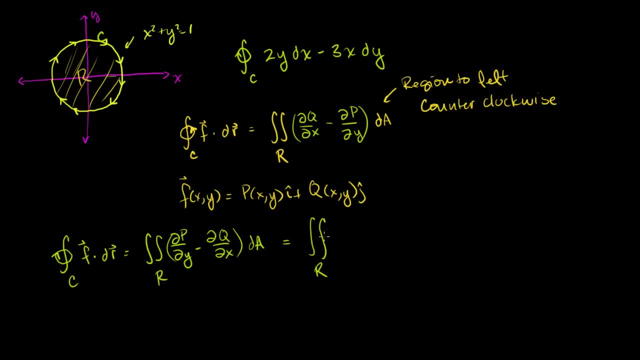 integral over the region. Let's just keep it abstract. for now. We could start setting the boundaries, but let's just keep the region abstract. And what is the partial of p with respect to? let's just remember this right here is our. I think we could. 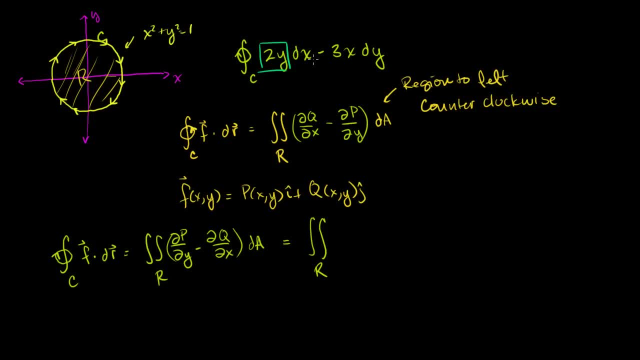 recognize right now that this: if we take f dot dr, we're going to get this. The dr contributes those components, The f contributes these two components. So this is p of xy, That is p of xy, And then this is q of xy. 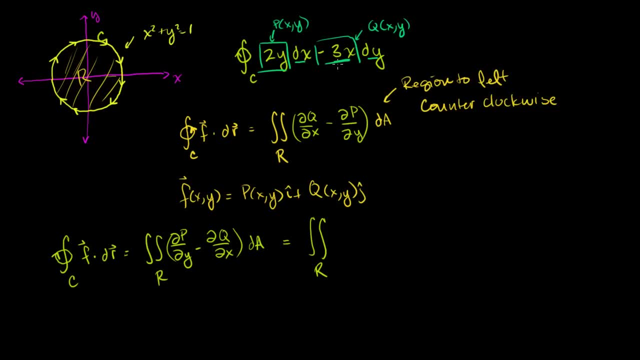 And we've seen it. I don't want to go into the whole dot dr and take the dot product over and over again. I think you can see that this is the dot product of two vectors. This is the x component of f, y component of f. 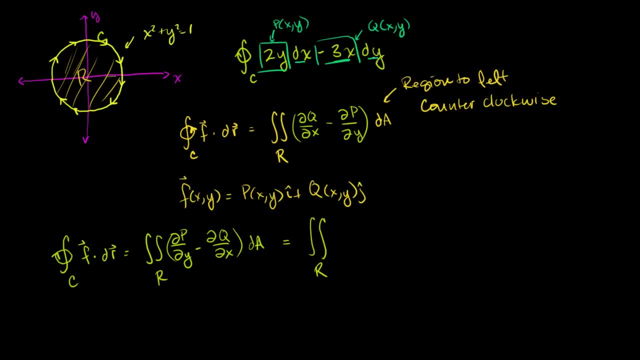 This is the x component of dr, y component of dr. So let's take the partial of p with respect to y, Take the derivative of this with respect to y. You get 2.. Derivative of 2y is just 2.. 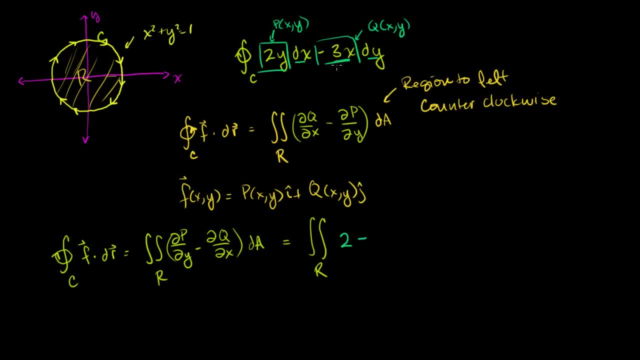 So you get 2.. And then minus the derivative of q with respect to x. Derivative of this with respect to x is minus 3.. So we're going to get minus 3.. And then all of that da, And this is equal to the integral over the region. 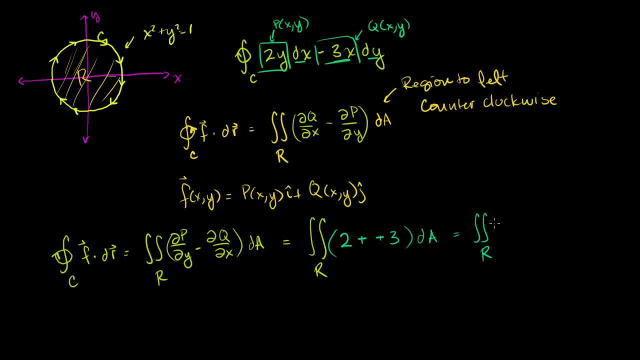 What's this? It's 2 minus minus Minus 3.. That's the same thing as 2 plus 3.. So it's the integral over the region of 5 da 5 is just a constant, So we can take it out of the integral. 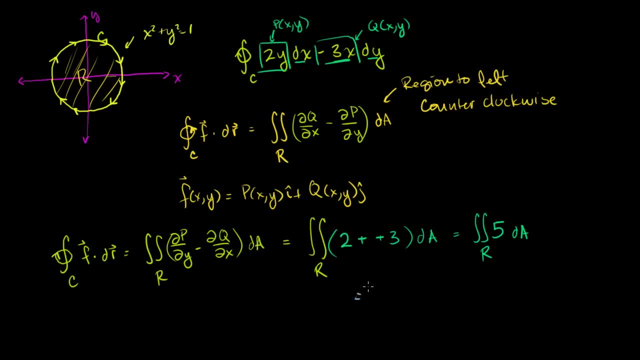 So this is going to turn out to be quite a simple problem. So this is going to be equal to 5 times the double integral over the region r da. Now, what is this thing? What is this thing right here? It looks very abstract, but we can solve this.